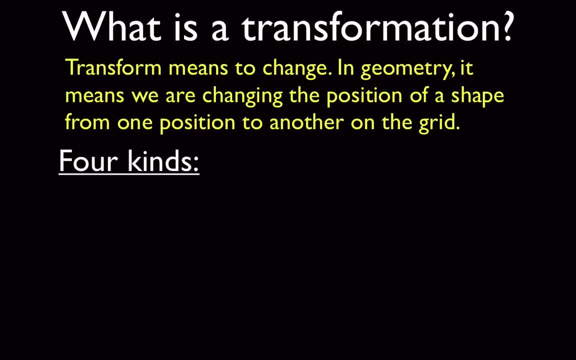 still change the position of all the points. So first off, we're going to talk about translations, also known as a slide. I like to think of it as when you're translating a word from one to another. it means the same thing, it's just in a different place, like a different language. 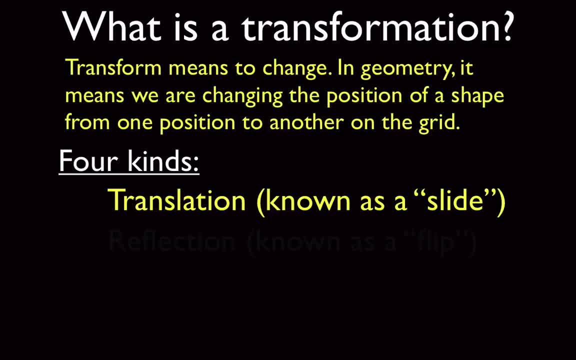 So that's what we're going to be talking about today, which is translations. You have reflections, which I think you know, reflection in the mirror, so that's a common one. We also call that sometimes a flip, because we're flipping over the shape and we're doing 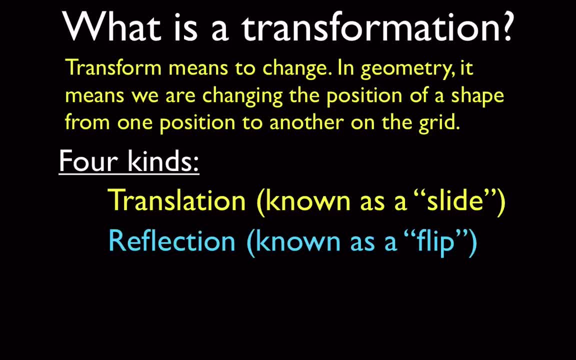 it across something like across the x-axis, across the y-axis, across a line can be done a lot of different ways: A rotation, which is also known as a turn, And, as you know, wheels rotate. rotation means to turn. 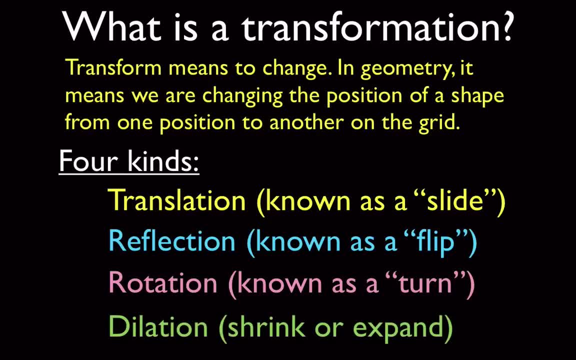 And the last one is a dilation. The first three, translation, reflection and rotation. those ones, they maintain congruency, because all we're doing is moving the thing, turning the thing, flipping the thing, but we don't change the shape and the size, which is, of course, the definition of congruence. 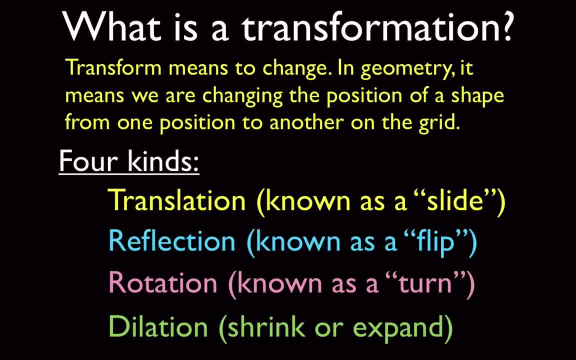 Same shape, same size. For dilation, we actually do shrink or expand the figure, so it keeps the same shape, but not the same size. For example, if we were to do a rotation, we're going to rotate the wheel and we're 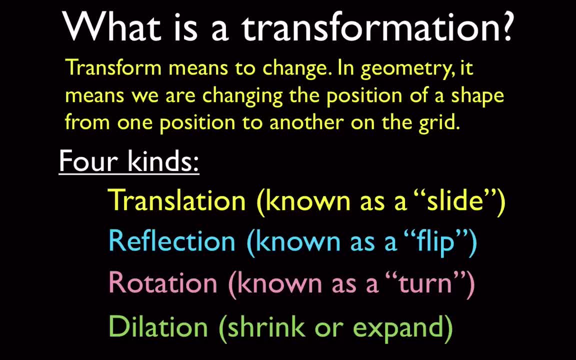 going to keep the same shape. For example, when you look in a mirror, it is a reflection, so it's the same image as you. it's just been flipped around. An example of something that wouldn't be like one of these four things would be like one. 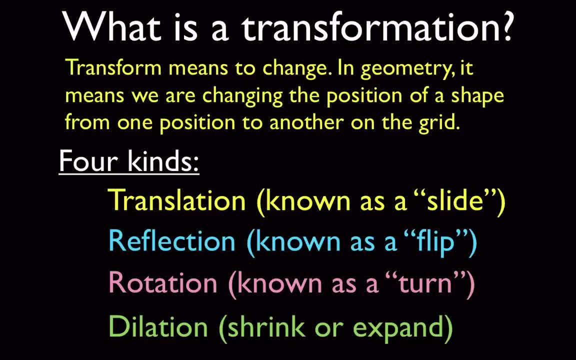 of those mirrors at the fun house, at the fair or the carnival, because the whole point of that thing is to make parts of you look bigger than other parts, And so it looks strange, it looks not normal, it's not similar or congruent. 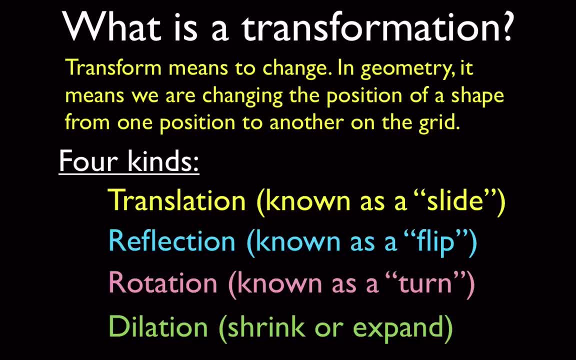 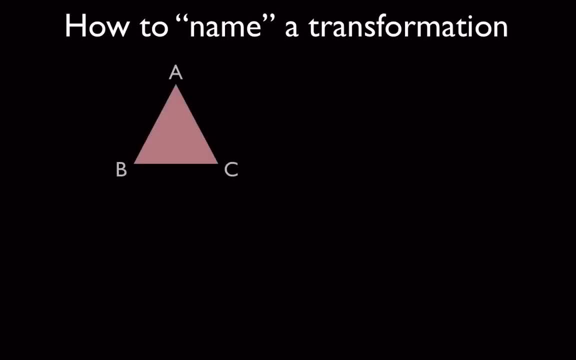 For all of these, we're either going to keep congruency, like the first three, or the last one will keep similarity And that the shape will stay the same. So, first of all, any time we talk about transformations, meaning we take the shape and we move the 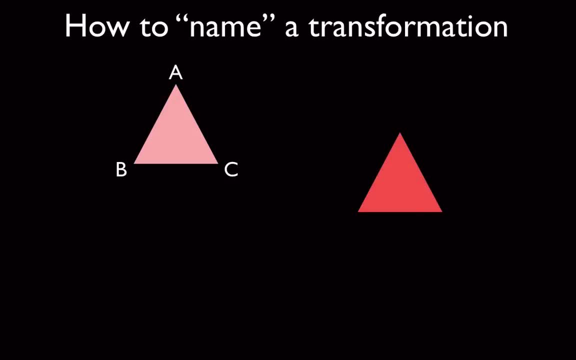 shape over to another spot, whether it's rotated or flipped or whatever, we don't just give it three new letters, We don't just go D, E, F or whatever. And the reason for that is we want to make a note that this is that figure just translated. 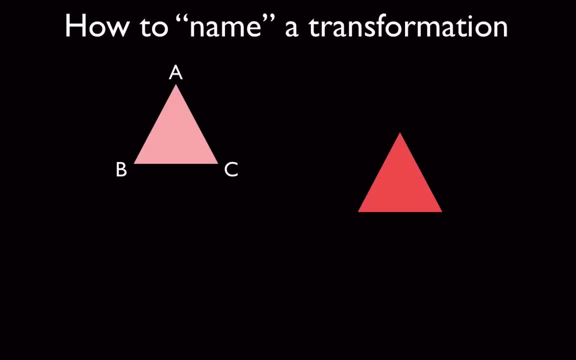 to another place in a mapping, a one-to-one mapping, so it's gone from one place to the next place. So what we do is we use the same three letters, But we put this symbol on them. that's called the prime symbol. 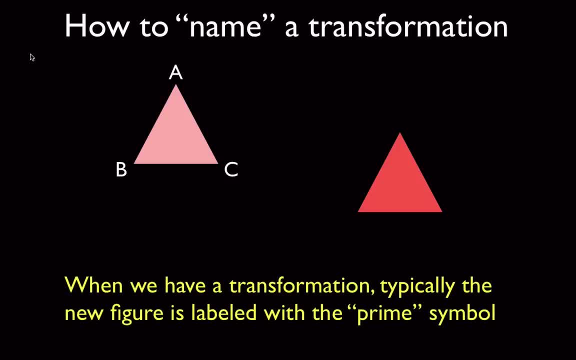 It kind of looks like a one, but it's not a one, it's more like a tally mark. So like that, If I had a second transformation, another one that we'd done from the original, I might use two tally marks, like A double prime, A triple prime for three, et cetera. 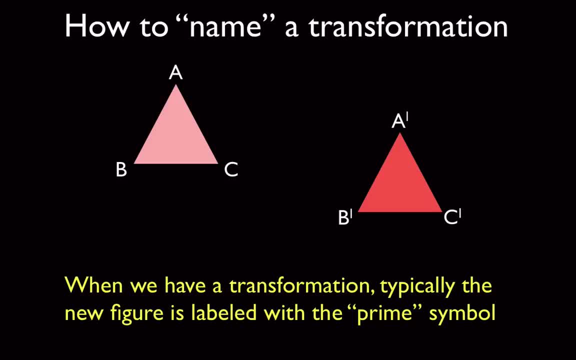 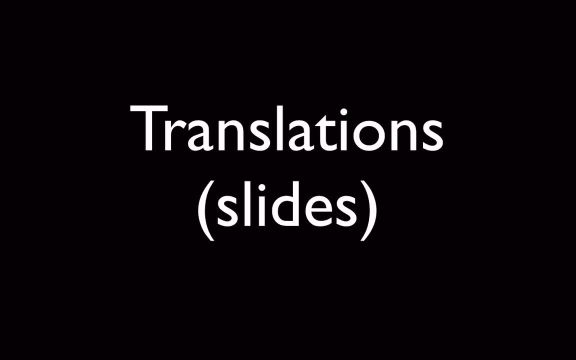 And so you just put extra marks on the thing, And what that shows is: that's where A went when we transformed it. that's where B went when we transformed it. that's where C went when we transformed it. Okay, what we're going to talk about today is translations. 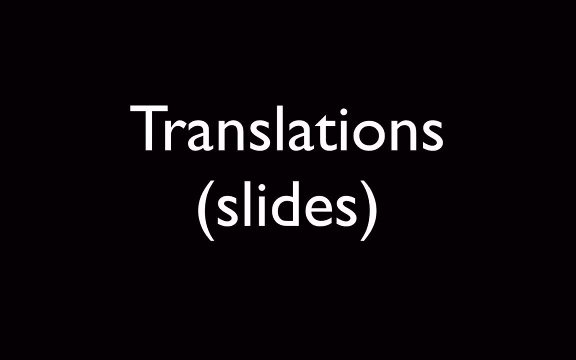 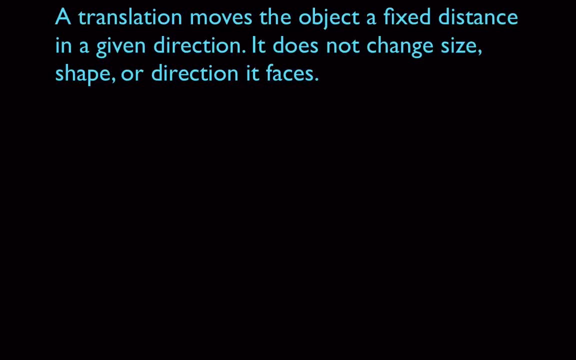 Okay, translations, remember, are slides going from one point to the next. So, first of all, a translation moves the object a fixed distance in a given direction. It does not change size, shape or direction it faces. So you're not going to have it turn, you're not going to have it flip over, you're just 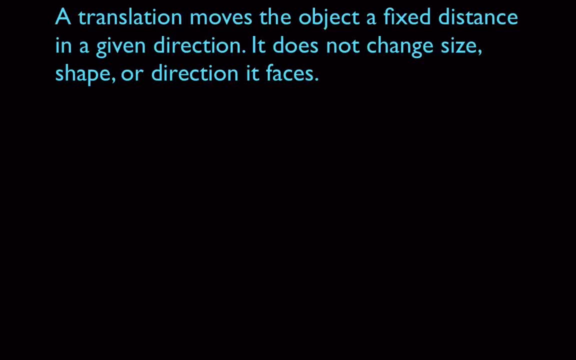 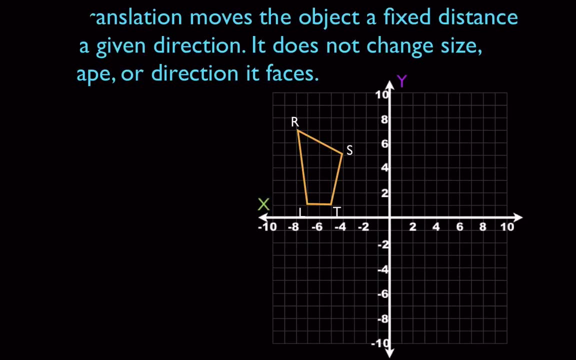 going to literally. it's like taking something on your table and sliding it with your hand without turning it, without rotating it. It's now in a new position, but it's facing the exact same way. Let's look at a specific example. okay, and this is ones already in your notes. 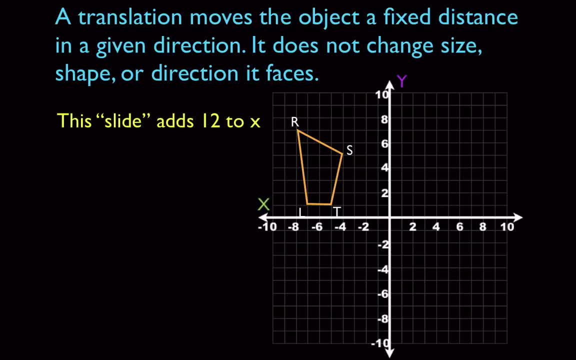 What we're going to do here is we're going to translate or slide 12 to X. So what that means is for every one of those four points, you see, and every point on the line that's not a labeled point- that whole thing is going to slide 12 to the right. okay. 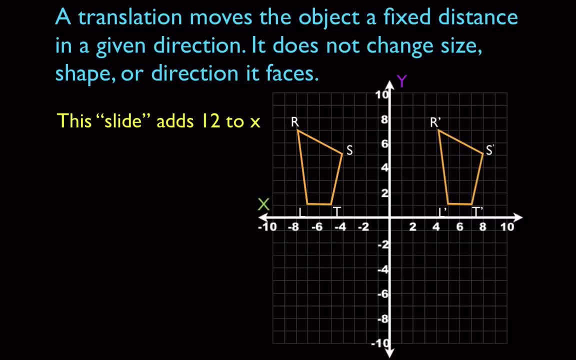 And so it looks a little bit something like this: Okay, So, as you can see, My negative seven now is at five. My negative five for T now is all the way over at positive seven. At S, I was at negative four and now I'm at eight. 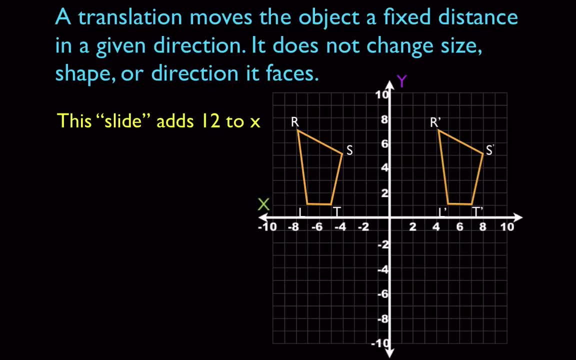 And for R I was at negative eight. now I'm at negative four. So everything is moved over 12 to the right. So a lot of people will ask: how do you do this? How do you easily do this? Well, there's a couple ways. 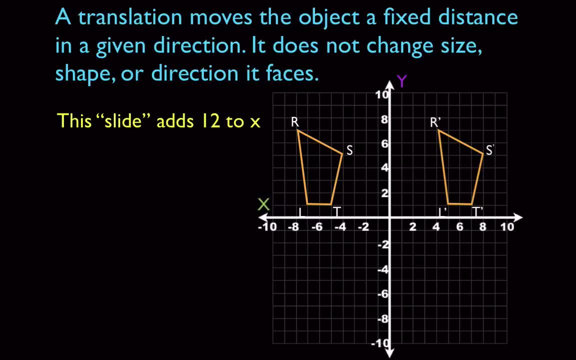 First of all, you could write down the points R, S, L and T. write them out as points, Okay, And then you could simply add 12 to all the X values and then draw your new figure. That would work just fine. 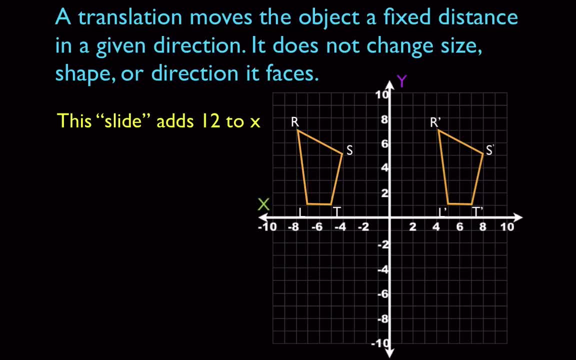 The second thing you could do is you could take each point, R, S, T, L and just count 12 over to the right and plot the point. That would work fine too if you did that and then connected the dots. 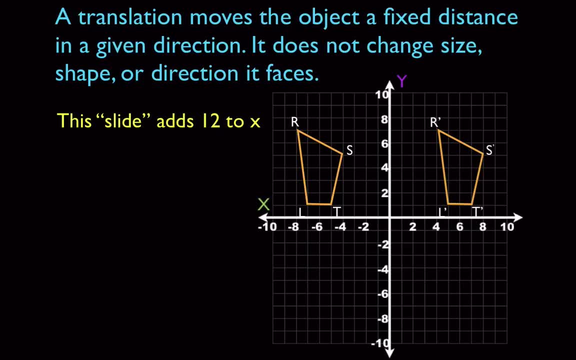 A third way- the way that I did it when I was a student- is to pick one point, Like, for example, if I pick S here, I go 12 over to the right and I put my point okay, And then all I would do is to get R. I notice that I go four to the left and two up, like 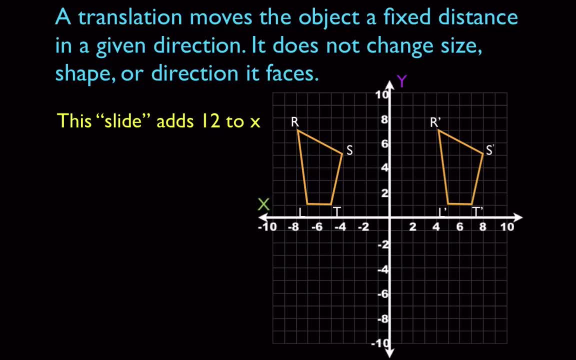 almost like make a little right triangle in my head And then for maybe T I'd go down four, left one And then two to the left of that would be L. So I basically use one point as a point of reference and compare all the rest of them. 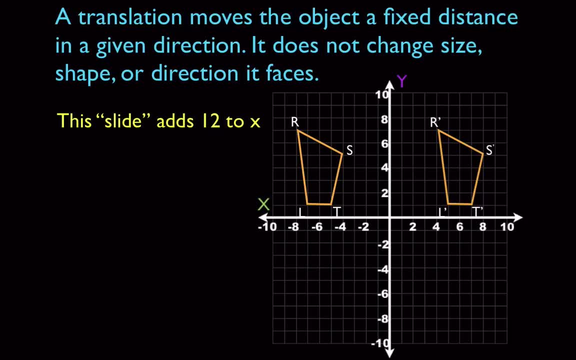 There is no right or wrong way. any way is correct, as long as you understand that each piece has been moved, the same amount, Even the points that aren't labeled, like the one right in between R and S. you can kind of see that crosses at a point there. 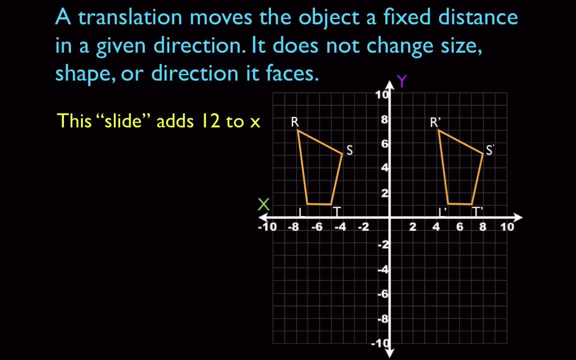 That, if you notice, is also exactly 12 to the right. If any one of them didn't move the right amount, we would lose congruency, meaning they wouldn't be the same size and the same shape anymore, And probably what would happen is it would look weird. 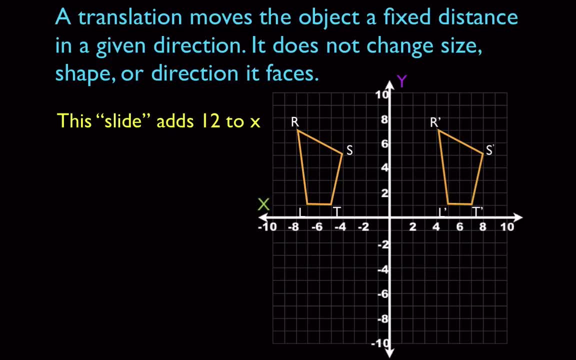 Something would look off. One of the things I do- I do notice my students do sometimes- is they do this too quickly and they'll count 11 over instead of 12 over for one of the points, And the shape's pretty close to the same, but it's not quite the same, so they maybe. 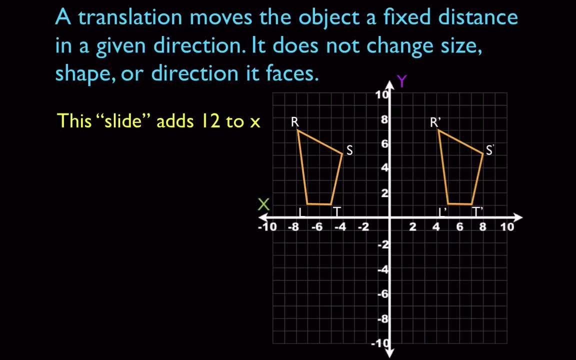 don't notice it. Unfortunately that would be incorrect on the test or something. So what you want to do is maybe have more than one step, So count to make sure there are 12 over, but also kind of count, you know, down to over. 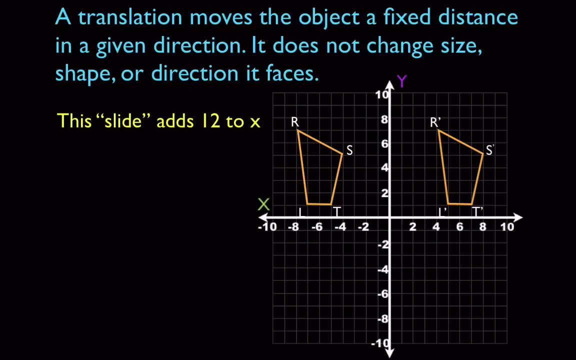 four to get from R to S and double check. those things still hold true as well. So the next thing I want to say is: how would this look? So I may say, hey, Slide by adding 12 to X, or do a translation by adding 12 to X. 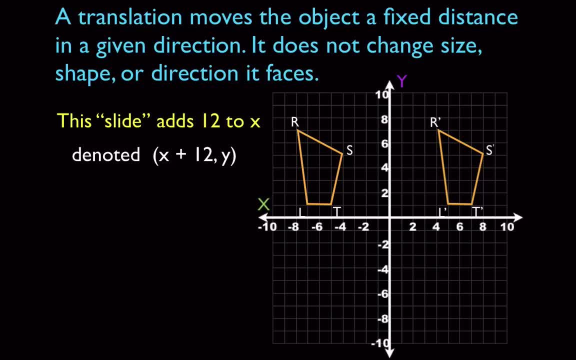 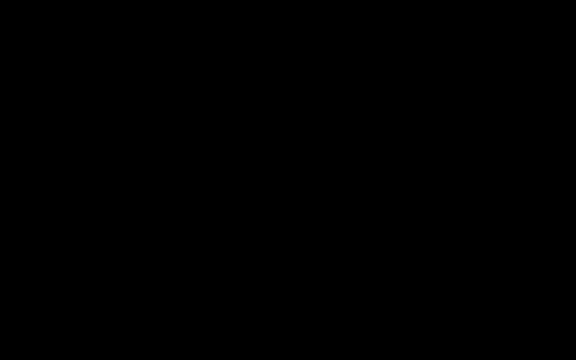 However, you may also see sort of like this: I want you to do the translation: parentheses: X plus two comma Y parentheses. What that means is it says: take X and add 12 to it, but leave Y alone. Okay, the next thing we're going to do is this is sort of like a two-step translation. 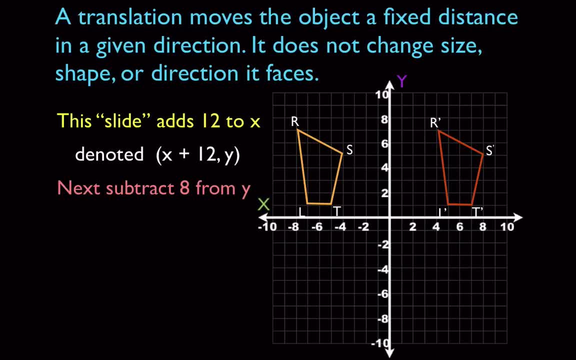 You can go ahead and put both of them on your paper. but if I were to do this two-step translation, usually what you would do is have to go sort of from one to the next and then down to the third Position. So in this case I'm going to subtract eight from Y, which means I'm going to take that. 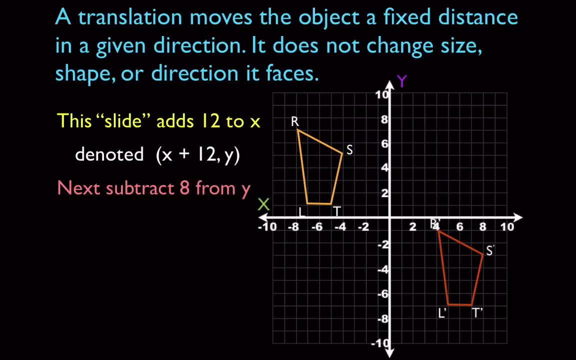 thing and I'm going to move every one of those points down by eight. Seeing it one more time, I'm going to take each of those points- I'm starting off at seven- and I'm going to move it down to negative one for our prime. 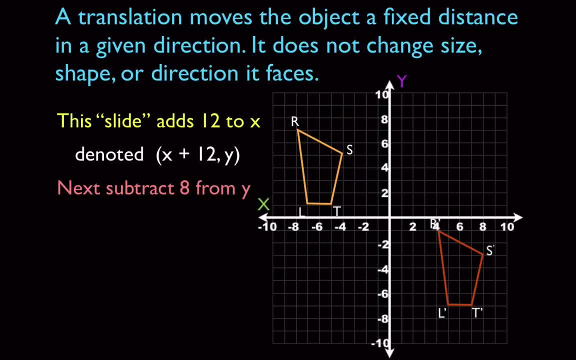 So at this point, again, same thing. I could have just taken each of those points I just had and subtracted it. Now, this translation you see right now is actually the translation X plus two, Y minus eight, because I did two things. 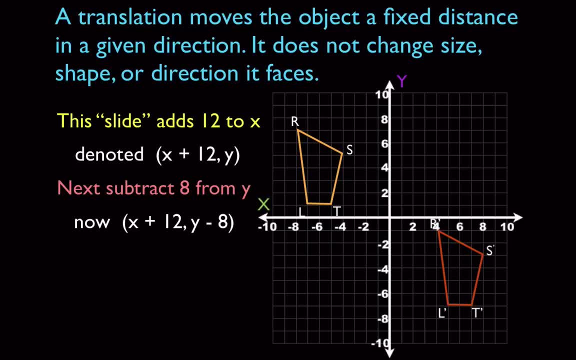 I moved to the right 12 and I moved down eight. Some of you might be wondering: could I have moved down eight first? Sure, Think about it. If I move down eight and then I move to the right 12, I'll be in the exact same position. 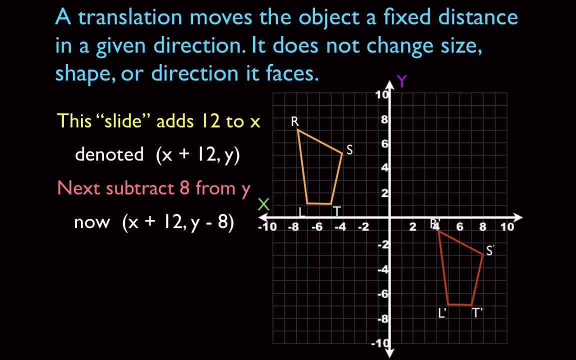 So it doesn't matter which one you do first. You might want to be a little bit careful when we start getting into flips and stuff like that, whether or not that still is true, But for now, since all we're doing is just sliding twice, it doesn't matter the order. 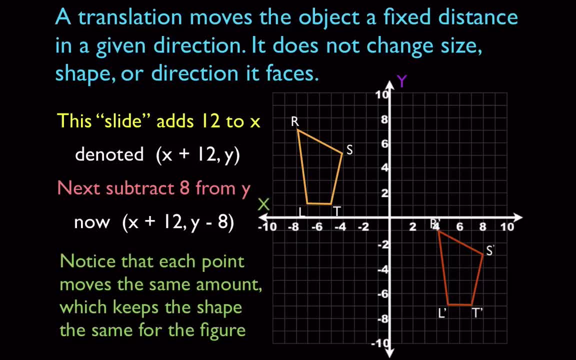 What I want you to pay attention to is, like we said, each point moves the same amount, which keeps the same shape for the figure. So why is this keep congruency? Because when you move every point at once, it doesn't change the shape, and it certainly. 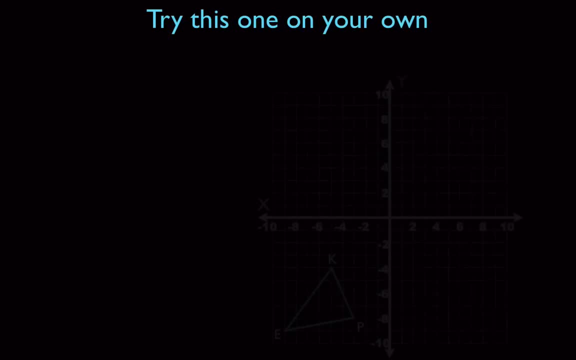 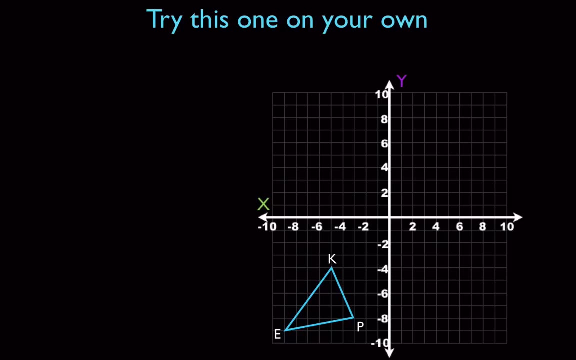 doesn't change the size. Okay, So this is the first example, So it may already be on your notes, but if not, you need to plot those- the K, P and E points on your on your paper, And we're going to do a few different things. 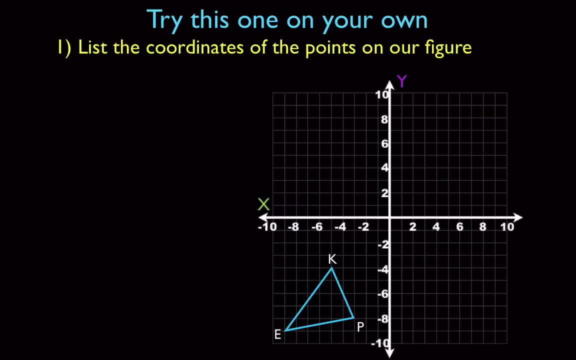 Okay, The first thing I'm going to have you do is I'm going to have you list the coordinates of the points on your figure. So by that I mean the actual points. So if you want to pause the video while you do that, that works. 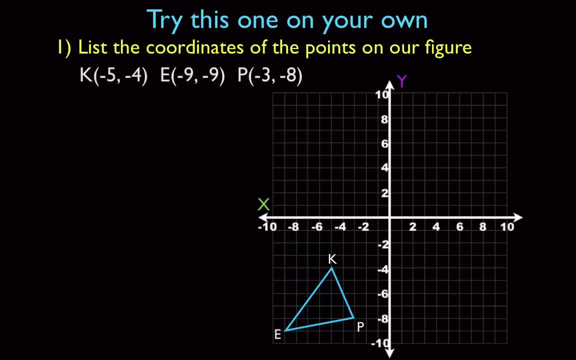 Okay, So the three points are negative. five comma negative four negative. nine comma negative nine, That's E- and negative three comma negative eight. Second thing we're going to do is we're going to do a translation, and the translation here. 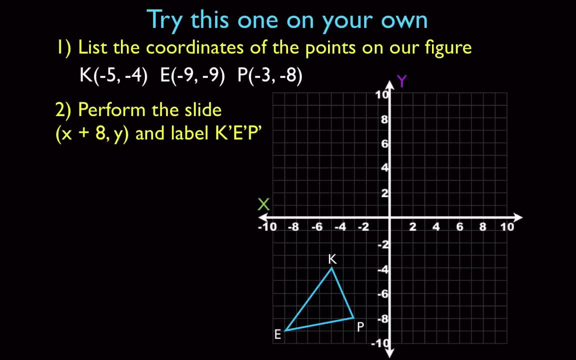 Okay, Add eight to X and only X, and not do anything to Y. So when you do that, go ahead and try that. Okay, Draw that on your paper label. it K, prime, E, prime, P, prime, and then hit play and we'll. 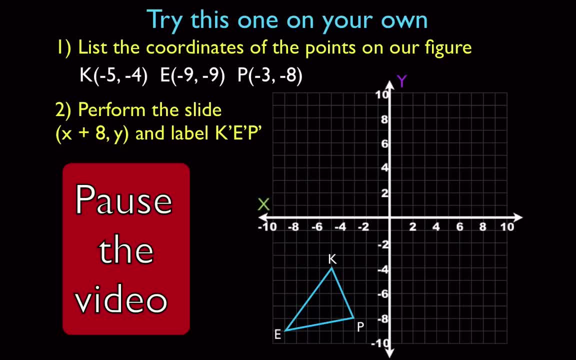 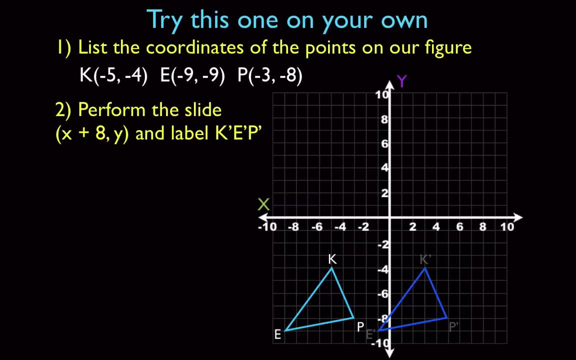 see if you have the correct figure, All right. So what should have happened is you should have ended up with that figure right there and you should have labeled it K prime, E prime and P prime. So, as you can see, I went from negative nine on the E point to negative one, et cetera. 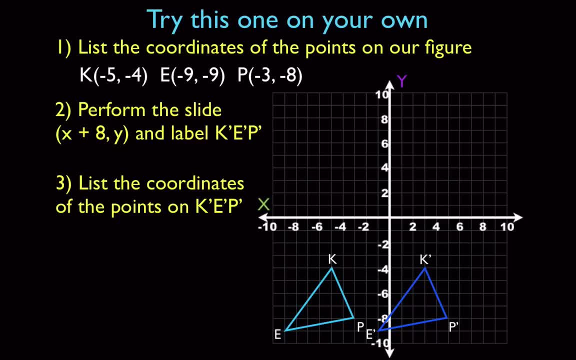 So now what I want you to do- the last thing- and you can pause it again- is list the coordinates of the points on KEP. Okay, So what you have here is hopefully what you realize is all I did is basically add eight to each of the Xs. 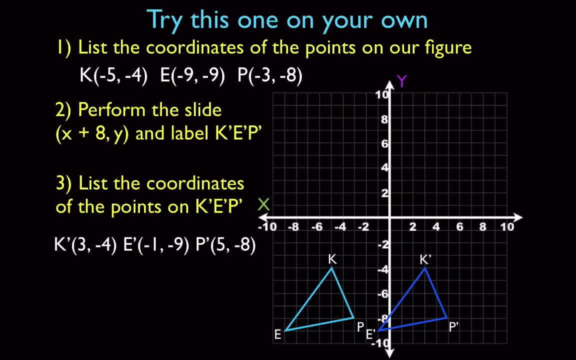 So the reason I had you do this is because you can see what we did is we actually drew the graph and then wrote down the points. but just as easily I could have written down my new points just by simply adding eight to each of the Xs and then went ahead and 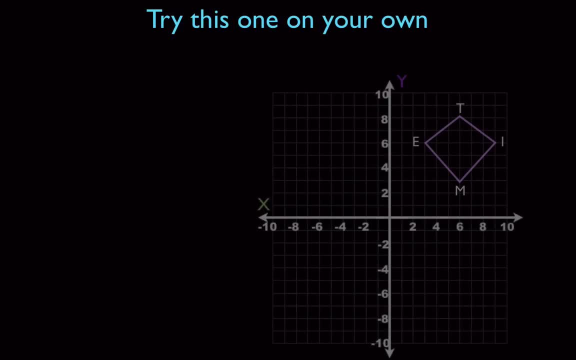 plotted those points. So again, that's just another way to do it. Okay, We're going to try another one. So go ahead and pause this for a second. Okay, So this is just like before. I'm going to have you go ahead and draw the figure on your paper and list the coordinates. 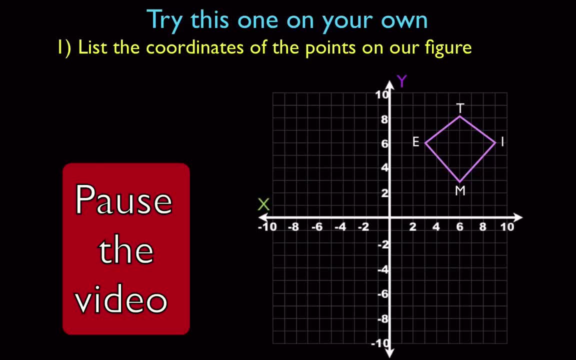 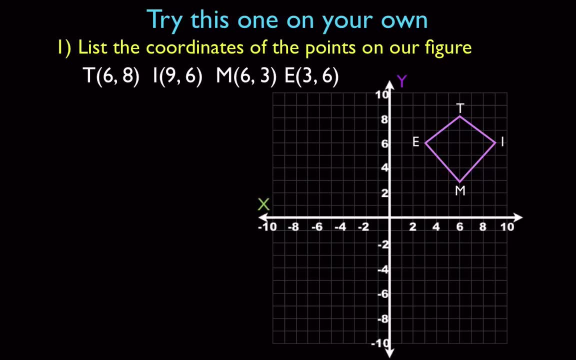 for each point. Okay, So if you did that correctly, your point should have been six comma eight, nine comma six, six comma three and three comma six. So you could see, because the E and the I and the T and the M are sort of diagonal or sorry. 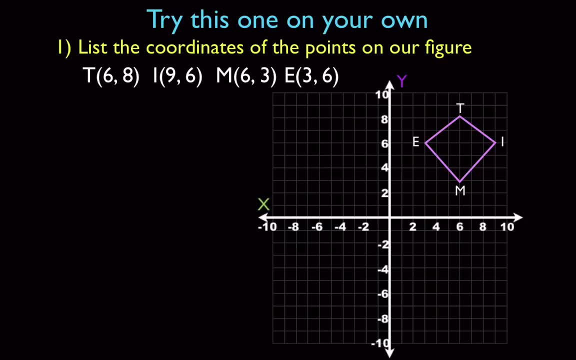 straight up and down or left and right from each other in that kite shape. there you get some of the same Xs and Ys This time. So the first thing I want you to do is I want you to subtract five from each of the Y values. 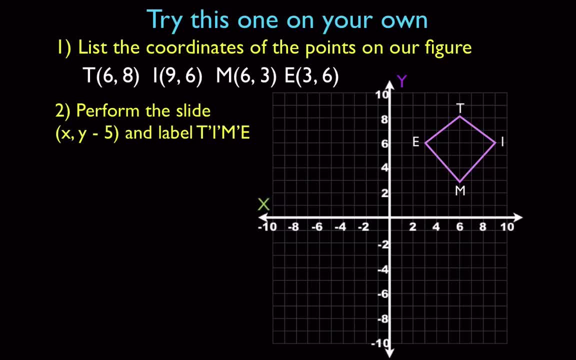 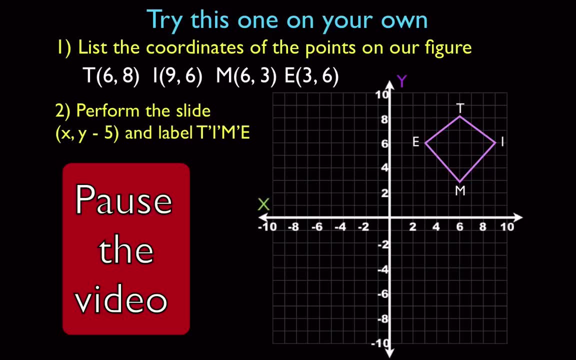 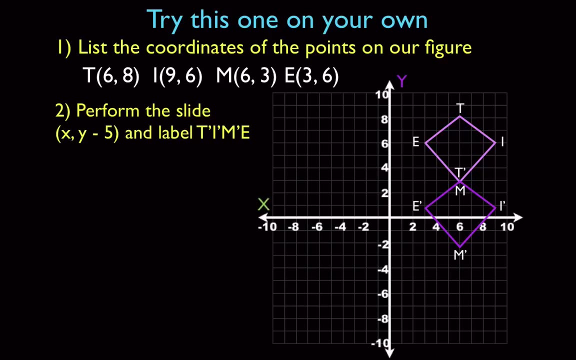 So we're going to perform a slide that is X comma, Y minus five, and label it T prime, I prime, M prime, E prime, All right, So you should have ended up with the figure right there, which is moving every shape down by five. 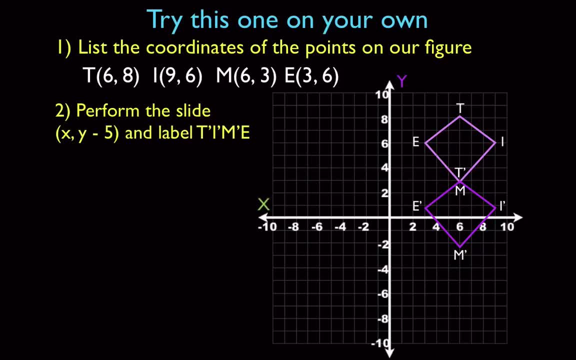 So from eight I went to three, from six for E I went down to one. Okay, And from I at six, I went down to one as well, Just like before. I want you to go ahead and pause it if you haven't done it already, and 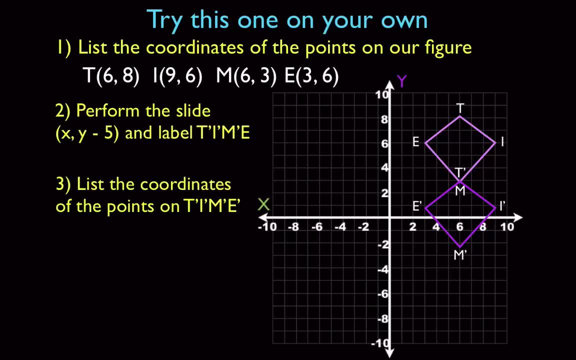 list out the coordinates for each of those points. Again, you should notice that you're just subtracting five from each of the Ys, All right, So hopefully you got this right. We subtract five from each of the Ys six, three, nine, one, six negative, two and three. 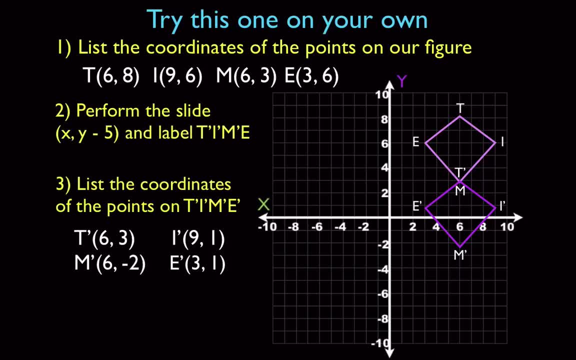 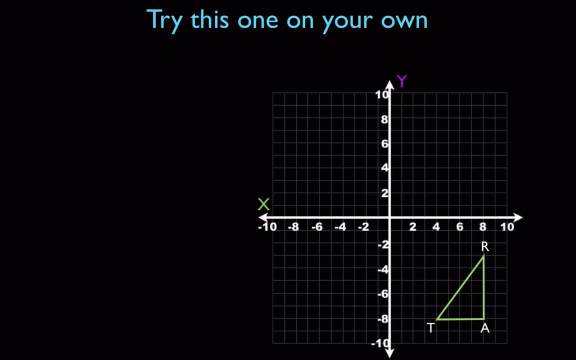 comma one, And hopefully you can verify that those points do in fact work on the graph. Okay, Let's try another one. So here you could see we have a what appears to be a right triangle, And I want you to go ahead first and draw the triangle and then list the points R, A. 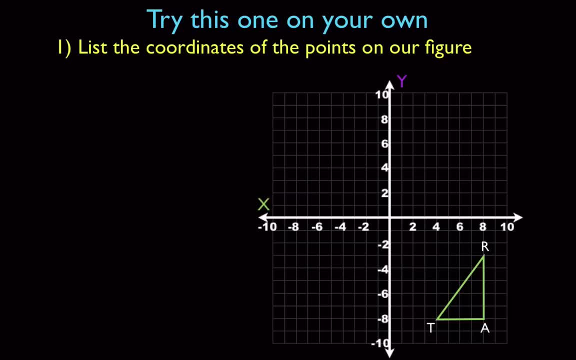 T as ordered pairs. Okay, So we're going to do now. the points are eight comma negative three, eight comma negative eight and four comma negative eight. Okay, So now what we're going to do is we're going to perform a slide or a translation that has: 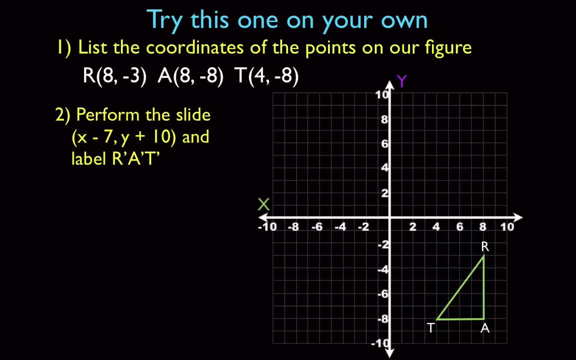 two parts. So we're going to subtract seven from all the Xs and add 10 to all of the Ys. So go ahead and do that. Make your translation. When you feel like you're good and done, go ahead and hit play. 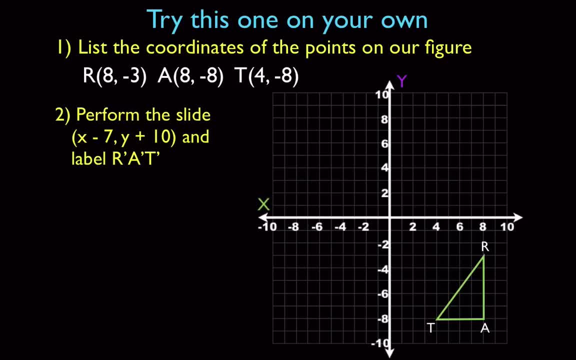 All right. So if you did it correctly, you should end up here And again, that is moving up 10 on the Y axis, So from negative three to positive seven And then moving over one, two, three, four, five, six, seven. 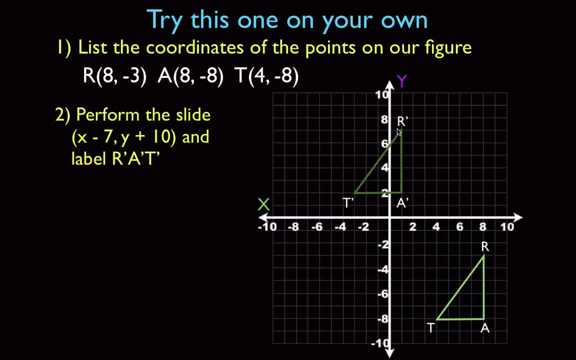 So, again, to do this in two steps, meaning draw the triangle and draw it a second time, to me is the hardest way to do it. You could look at it almost like slope, where you go up 10,, left seven, but I still feel. 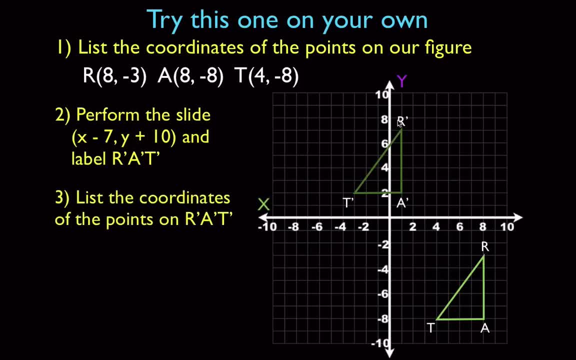 like. the easiest thing to do here is to simply figure out the coordinates of the R prime, A prime and T prime by subtracting seven and adding 10 and simply plotting your points on the paper. So go ahead and write those three points. verify that you did. 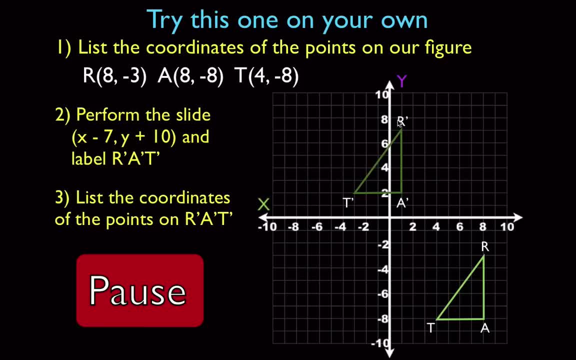 In fact subtract seven from each of the Xs, add 10 to each of the Ys and hit play when you're ready, All right. So hopefully you noticed we went from eight to one, which is subtracting seven, and from negative three to seven, which is adding 10..